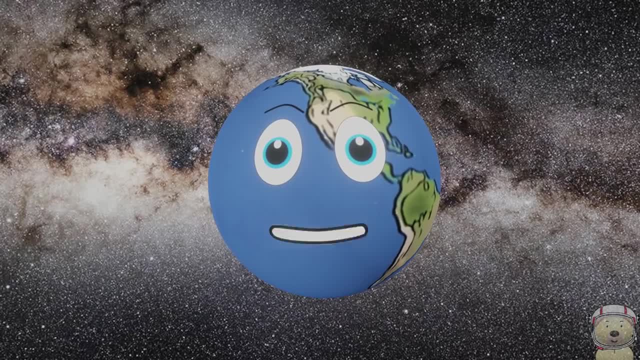 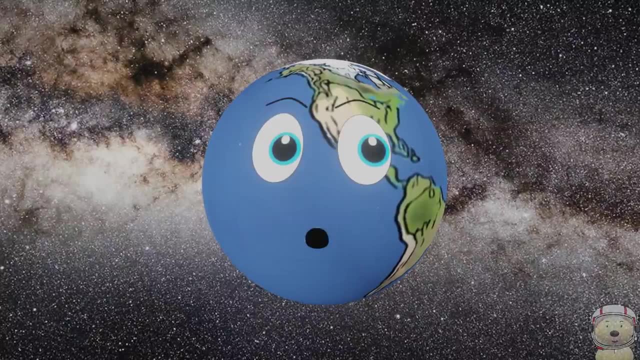 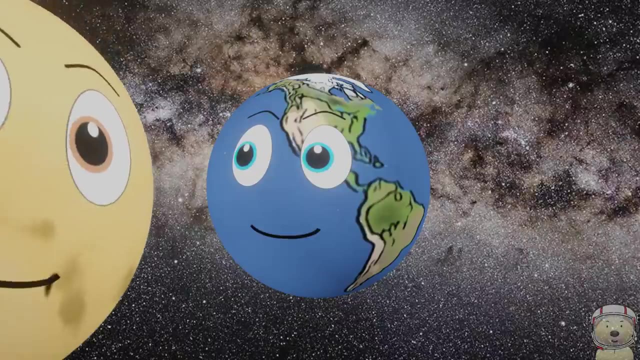 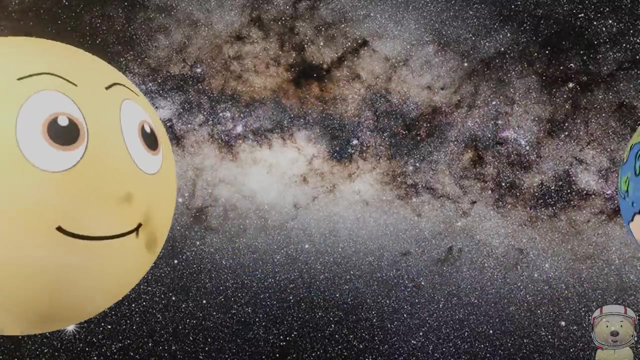 Hi, all, welcome to my video, Our video, Our video On planets and their moons. I'm planet Earth And this is planet Venus. Hi, let's go across the solar system and find a planet to talk to Venus. did you ring the camera? 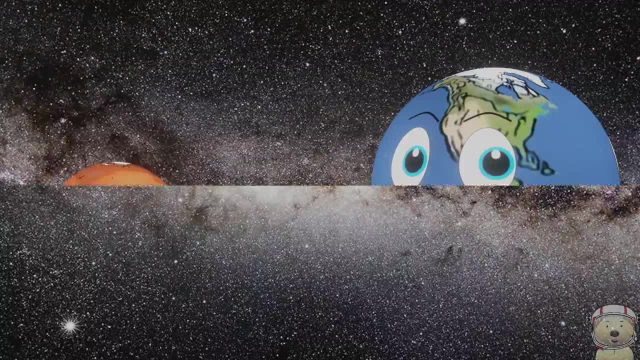 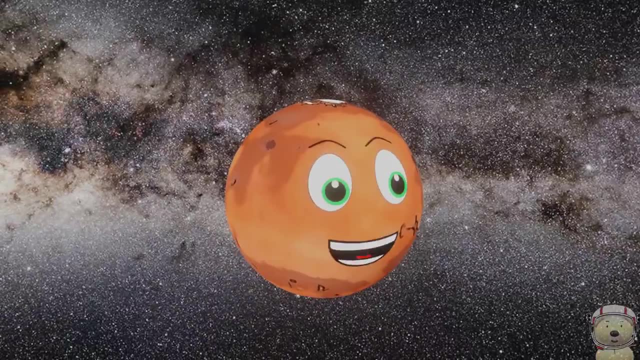 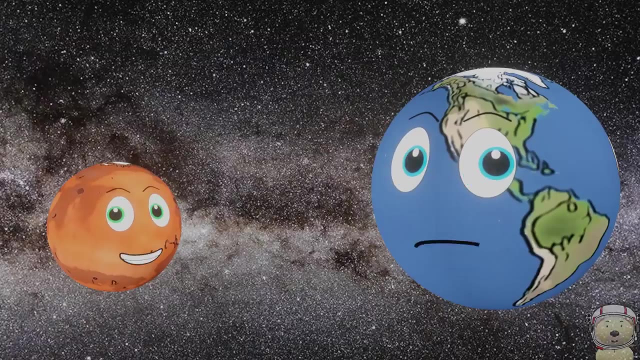 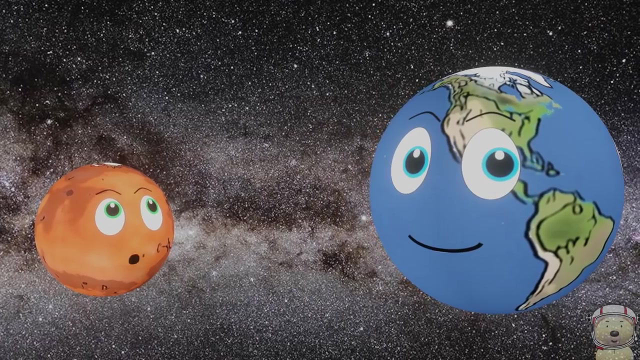 Here's our first planet. Hey, Mars, how are you? I'm great thanks Earth. How are you guys? I'm great thanks Mars. I'm annoying. Good Thanks Mars. We've come to talk about your moons, Mars Cool. 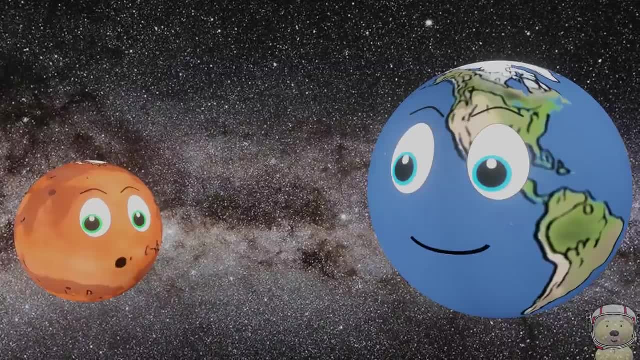 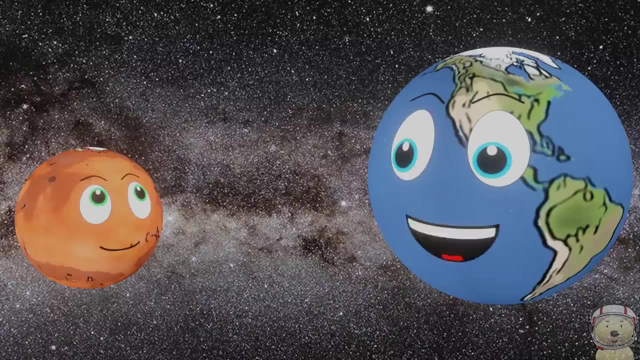 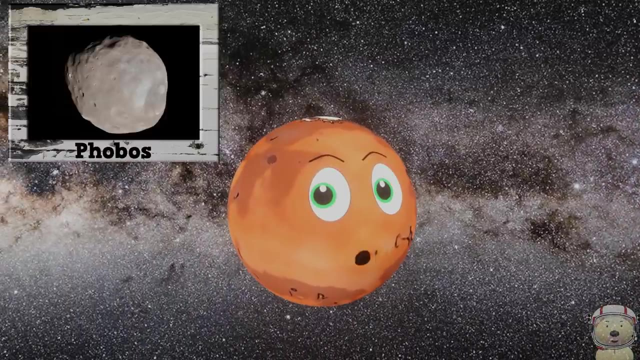 How many moons do you have? I have two moons. Two, That's all. What a waste of my time. So, Mars, you have two moons. That's so cool. Tell me about them. Well, they are called Phobos and Deimos and they are very odd shaped. It is possible they 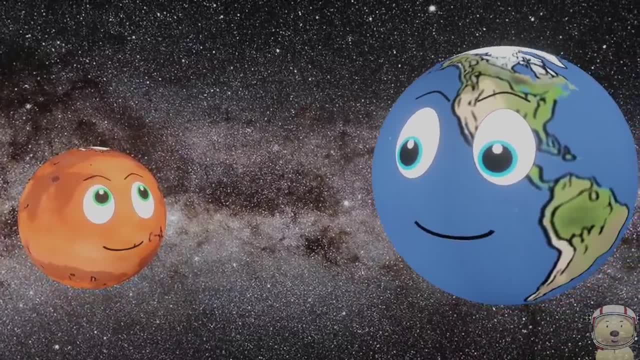 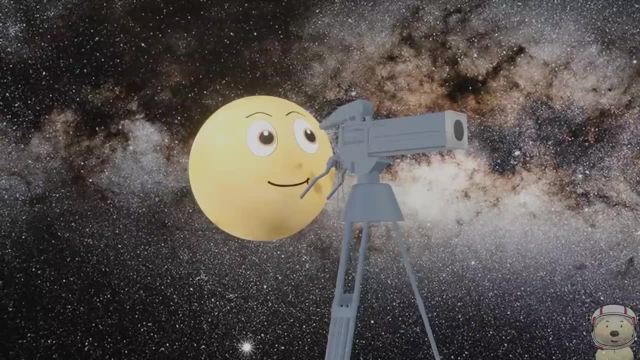 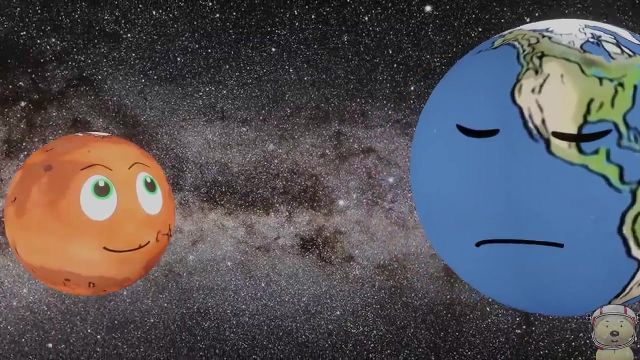 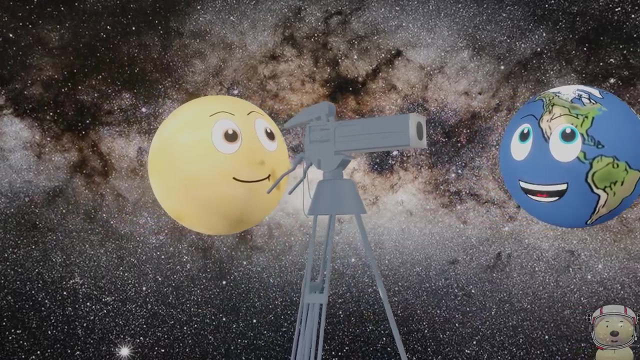 are asteroids left over that were captured by me. Great facts, thanks. Any more questions? Venus, Yes, What time is lunch? N-no about Mars. Well, thank you, Mars. On to the next planet: Lunch. Really, It's only 9am. 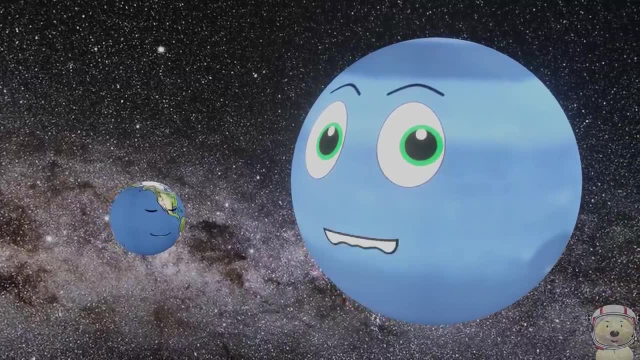 Next up: planet Neptune, Hey Earth, Hey Venus, Hey Neptune. Now, obviously you are known as the planet Neptune. Hey Earth, Hey Venus, Hey Neptune. Now, obviously you are known as the planet Neptune. Hey Earth, Hey Venus, Hey Neptune. 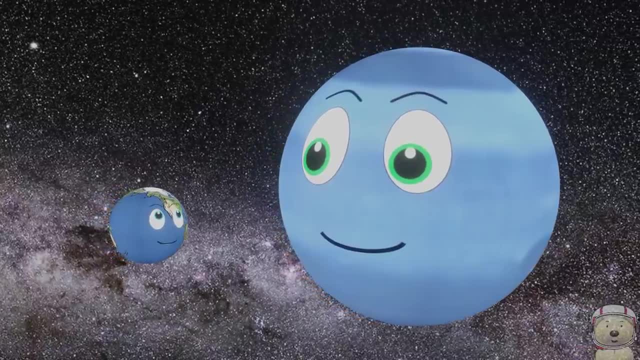 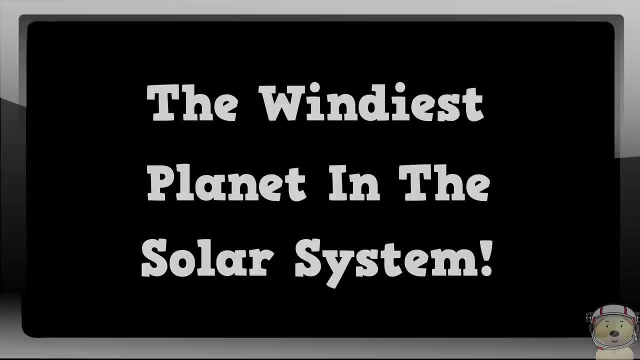 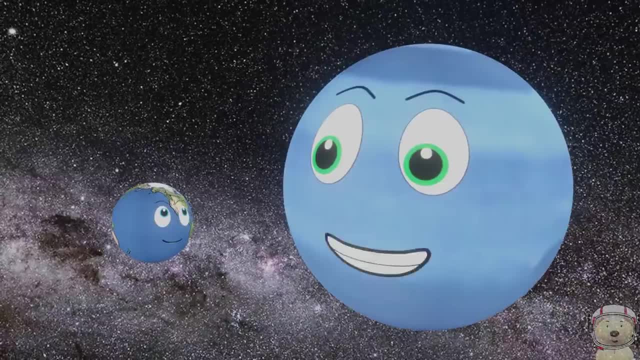 What are you doing, Venus? Nothing, But how many moons do you have? I have a lot of moons. I actually have 14 moons. 14? Wow, Is it a lie? What did you say? I want some pie. Oh, yes, we have 14 moons. 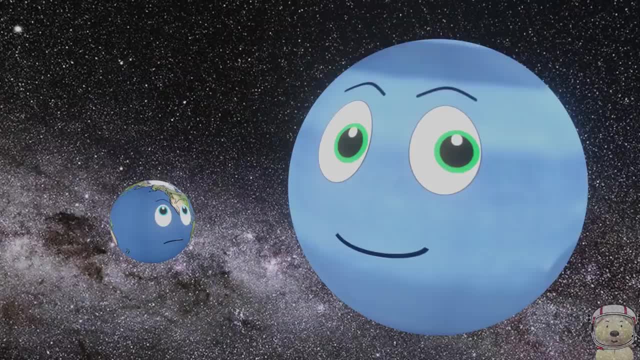 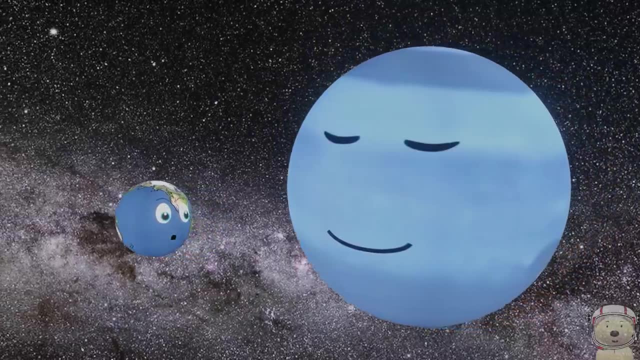 Oh, I see. I see, We have 14 moons. I love my moon. We have 12 moons And we have 14 moons. And who's next? Oh, yes, me too, I'm very hungry. Tell us something about your moons. 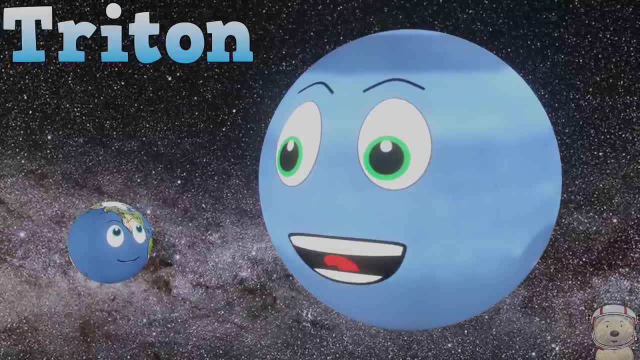 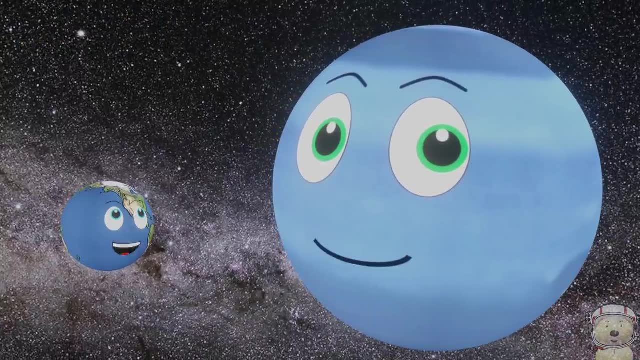 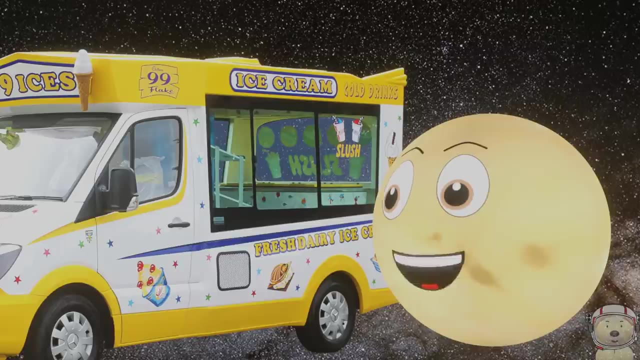 My largest moon is called Triton. It's a little bit smaller than Earth's moon, but it's covered in active volcanoes, Venus. do you have any questions, Venus? And can I also have an ice cream with chocolate sauce and sprinkles please? 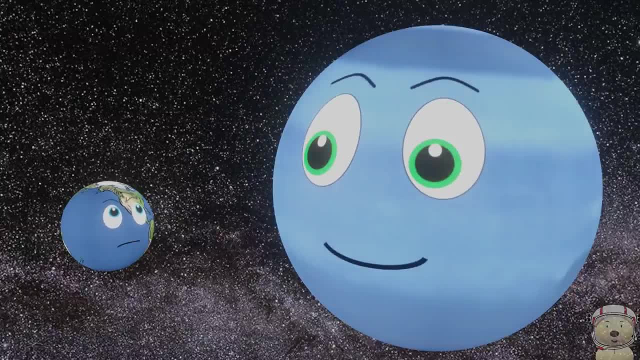 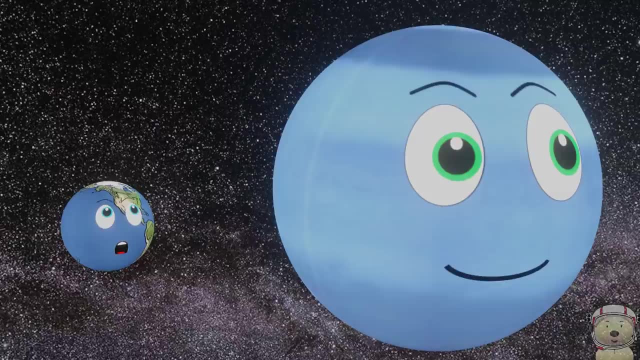 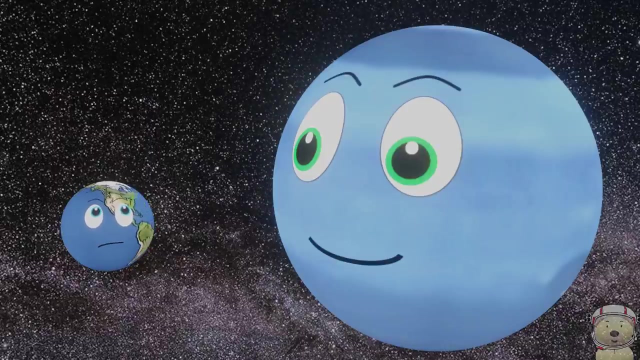 Venus. we're filming here. What are you doing? Ooh, ooh. can I have a rocket lolly please, And a rocket lolly please. This is so unprofessional. Can I get a strawberry cone please? 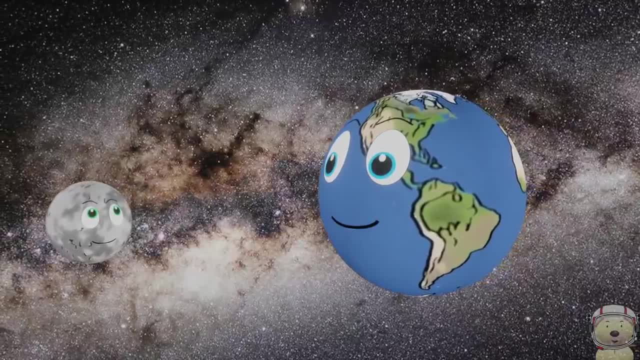 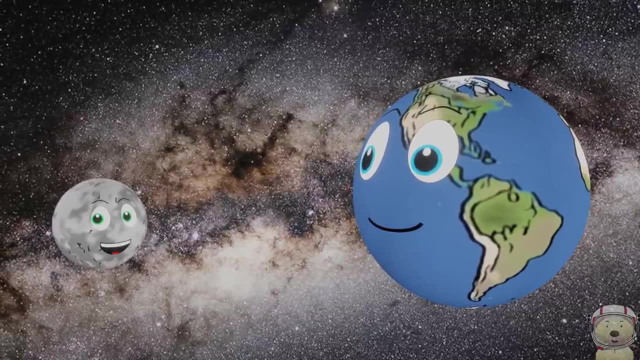 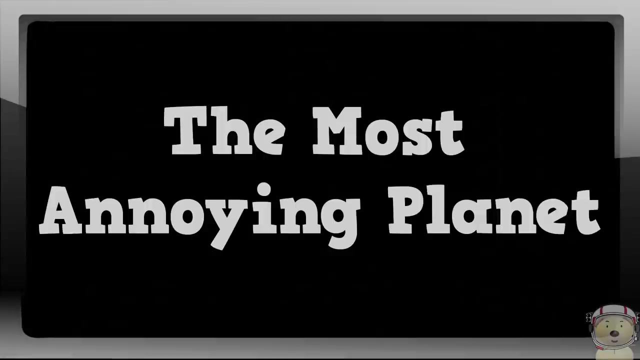 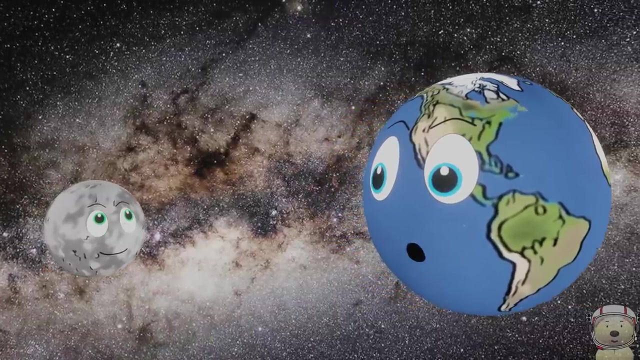 On to planet Mercury. How are you? I'm great guys. Oh, it's Venus. I'll only do this if she doesn't call me annoying again. Uh, okay, I promise, The most annoying planet, Venus. So, Mercury, how many moons do you have? 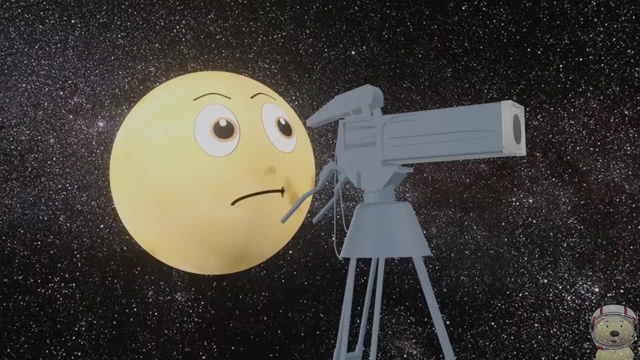 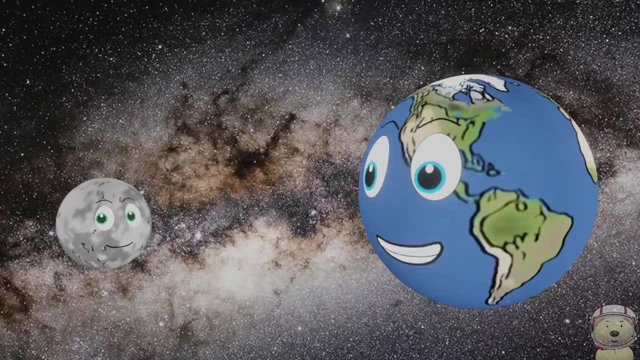 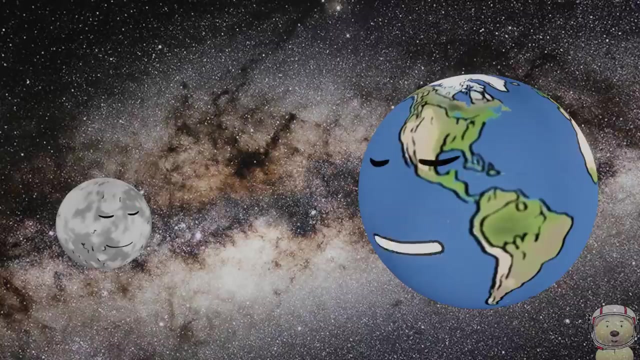 Uh, I have no moons, Great Shall, I pack up. then Hang on, hang on. What do you mean? you have no moons? He means he has no moons. No, I know that. but what I mean is why. 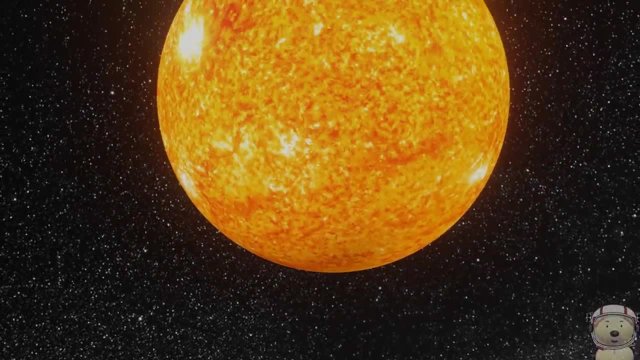 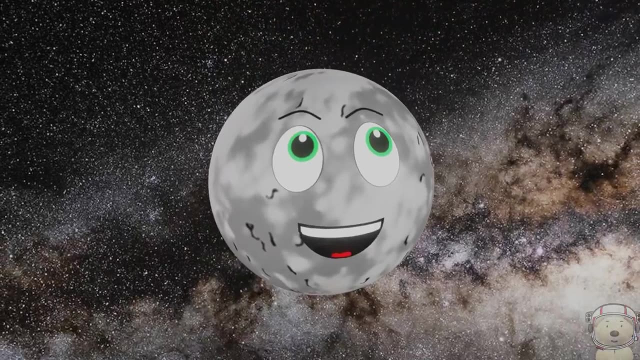 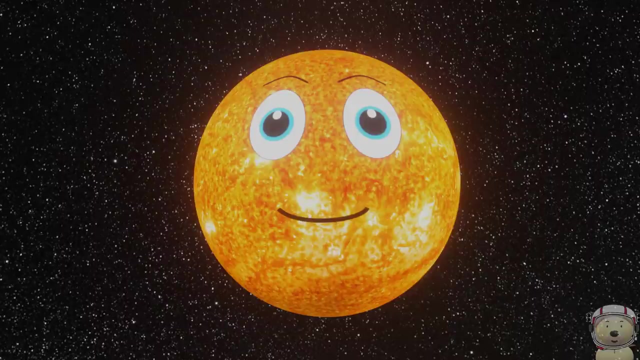 Well, because I am so close to the Sun and its gravity, plus I am so small I can't hold my own moons. Any moon I had would just get captured by the Sun. Oh, stupid Sun S Stupid Sun. 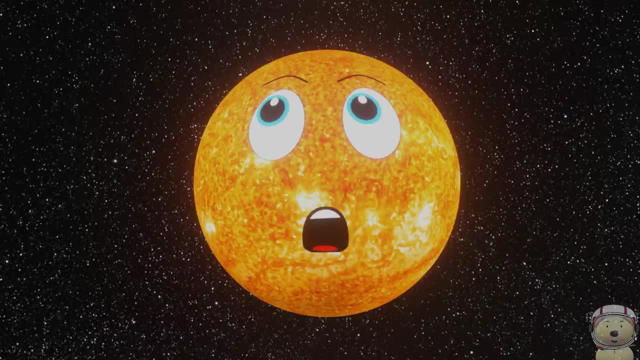 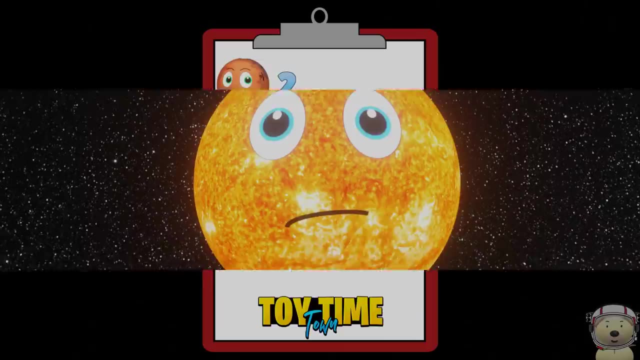 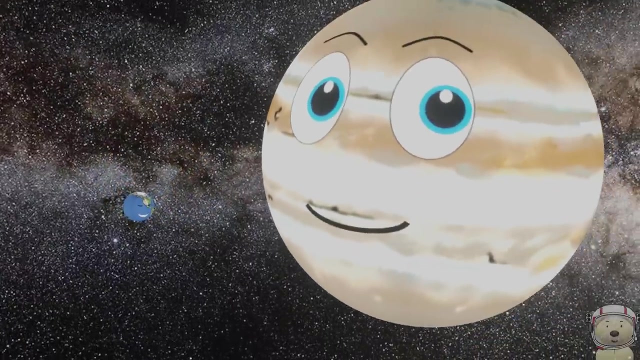 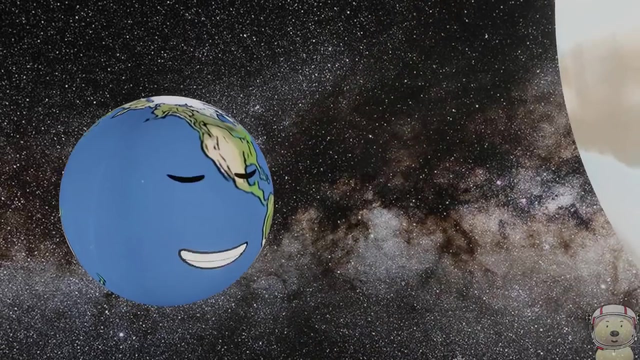 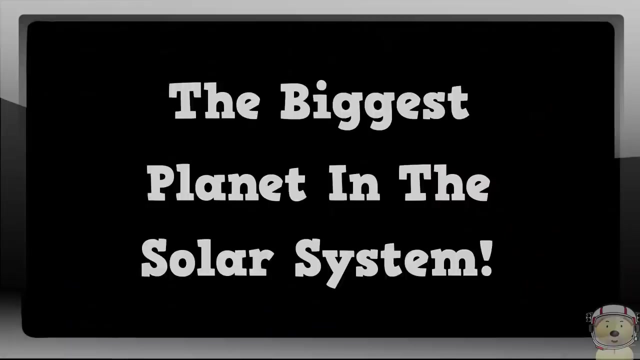 Stupid Sun S Stupid Sun On to Jupiter. Hey Big J, Hey guys, How are you Now, Jupiter? Now Jupiter, You are the BIG J, aren't you planet in the solar system, the biggest planet in the solar system? yes, I just. 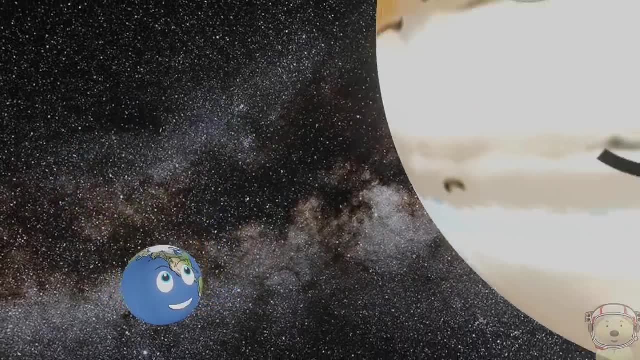 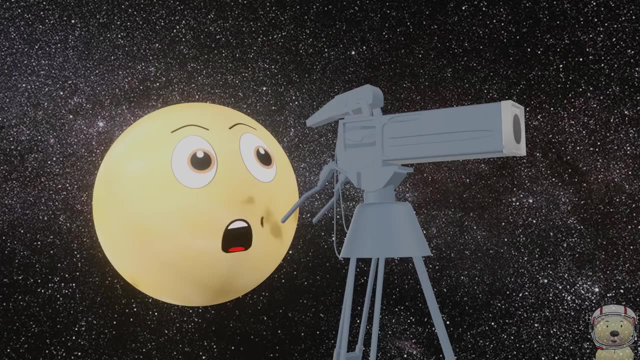 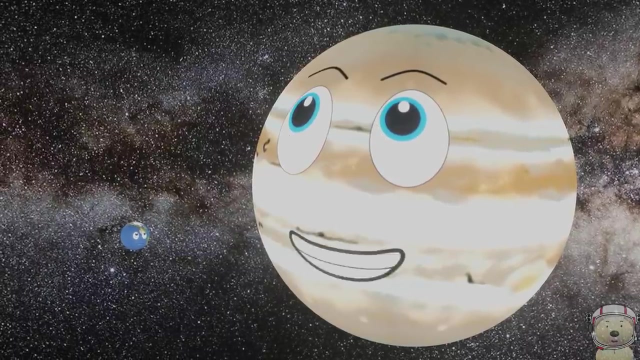 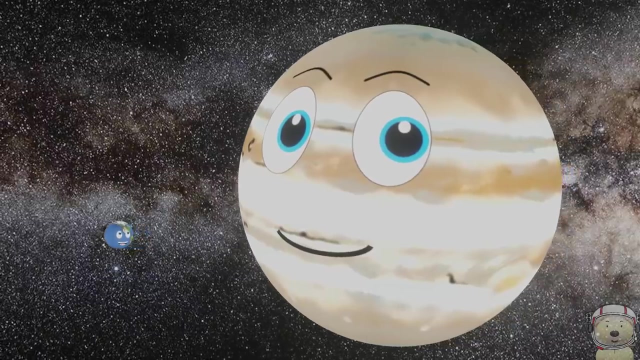 wanted to try it, but do you have a lot of moons? yes, I do. I have 79 moons, whoa, Wow, I also have the largest moon in the solar system, Ganymede. Ganymede is actually bigger than Mercury and less annoying. hey, that is incredible. well. 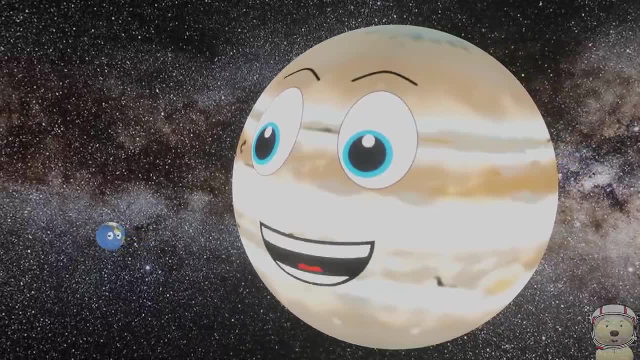 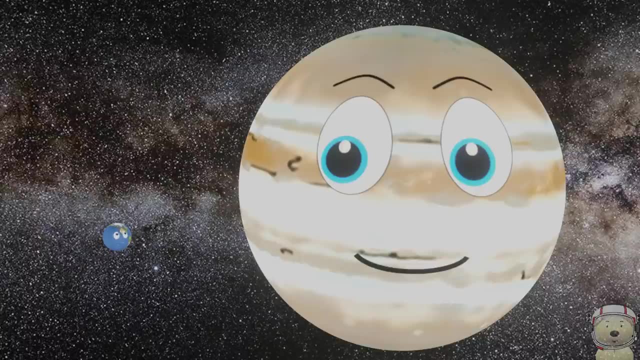 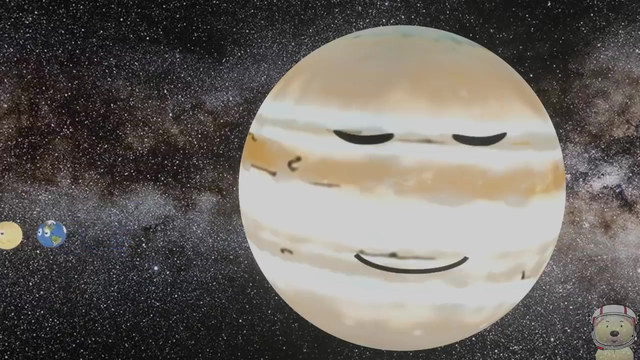 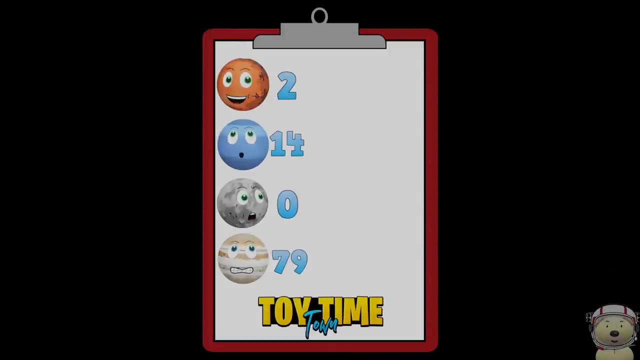 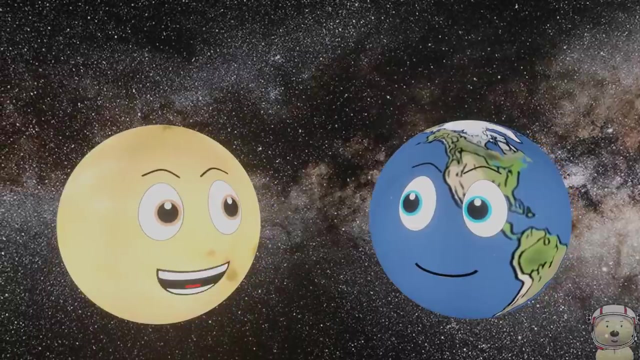 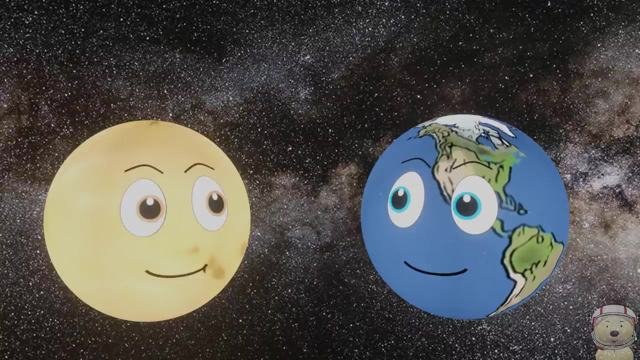 thank you. I'll tell you all of my moon names, shall I? well, there's Ganymede, Europa, Io, um, shall we go? yep, Callisto, Ursa, Kale, core. hey, I just realized we haven't had your moons Yeti. hey, hi, Venus, how many moons do you have it? well, 88, no, 80, no, wow. 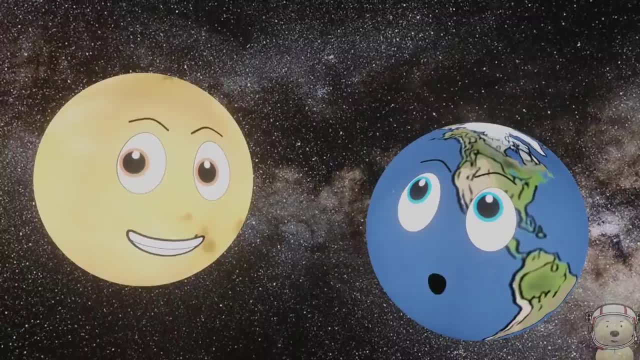 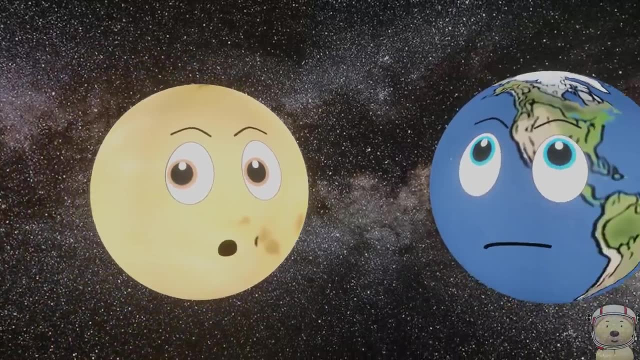 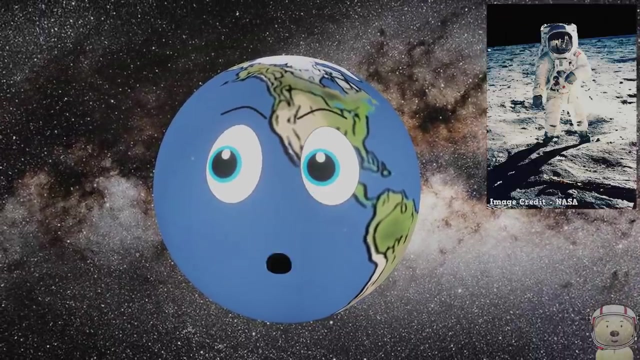 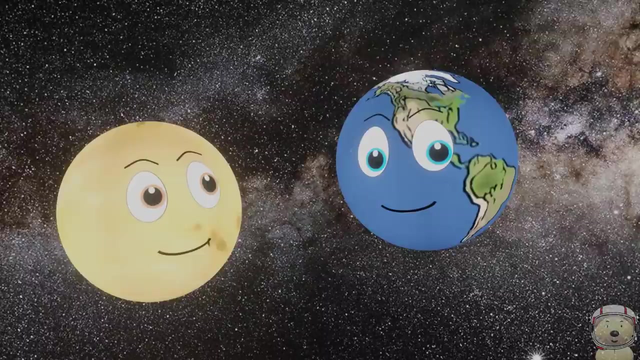 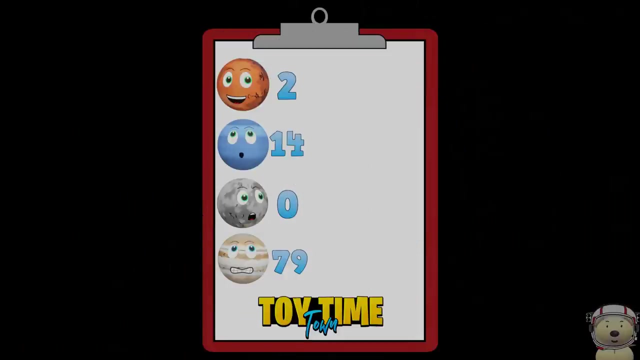 maybe 34 them? no, I, i have one moon, so sorry, how many one? wow, 100 moons. no, just one. but my moon is amazing because it is the only moon that humans have ever been on. that that's pretty much, it, isn't it? yeah, shall we move on? let's move on. 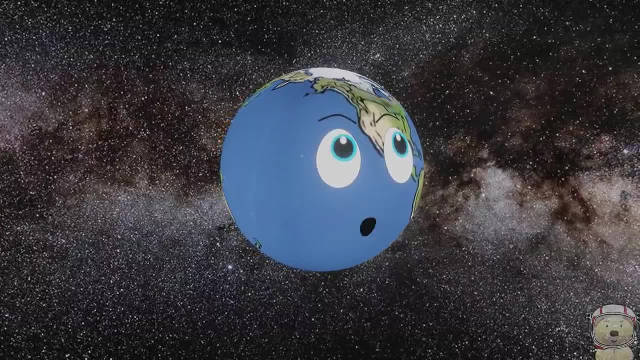 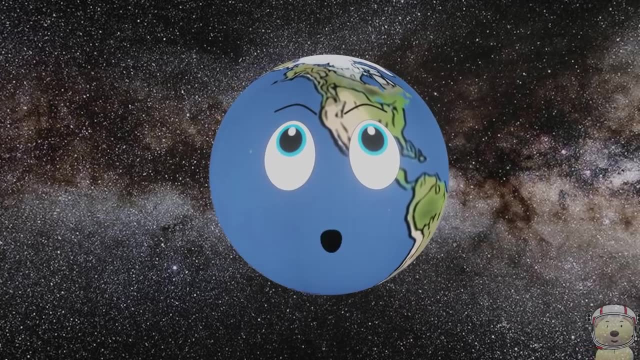 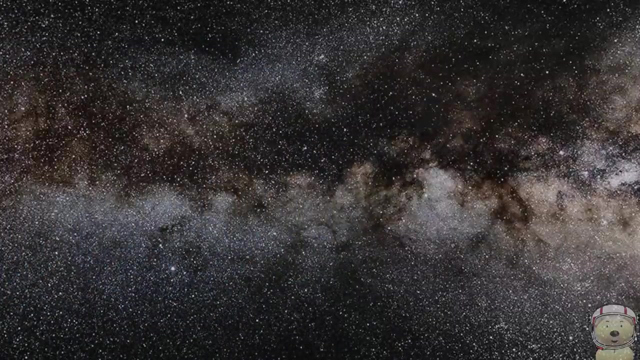 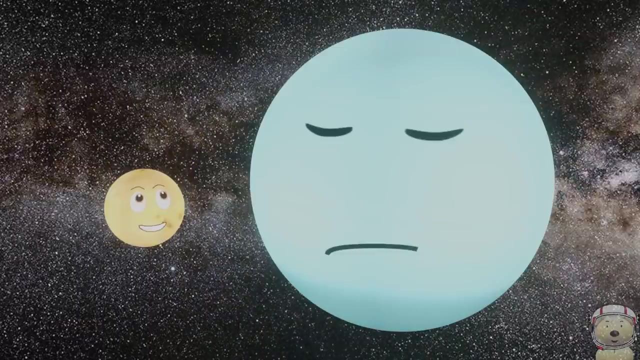 on the planet. uranus, venus, the lighting is not quite right here. can you turn the light up please? yes, sure, ah, too bright i can't see. oops, sorry, perhaps i'd better take over. hey, uranus, hey venus, we're here to ask: how many moons do you have? 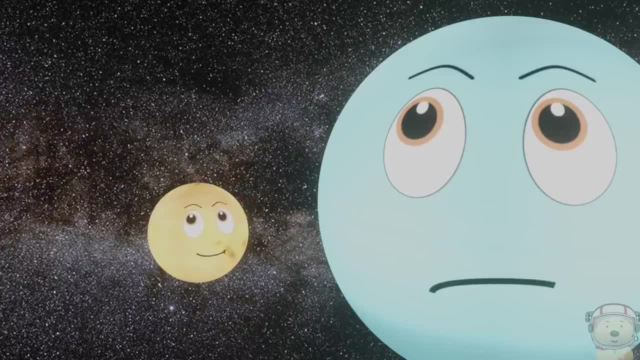 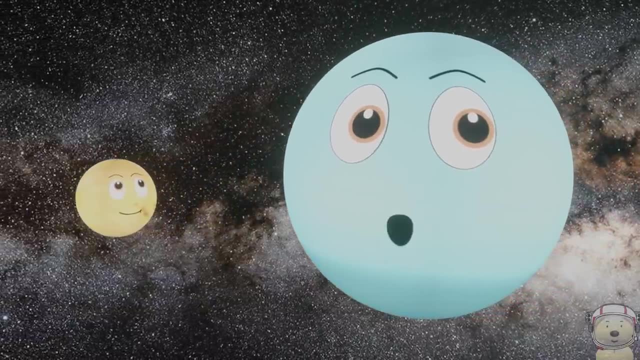 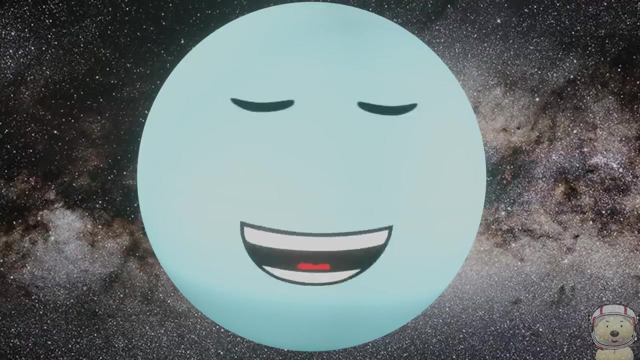 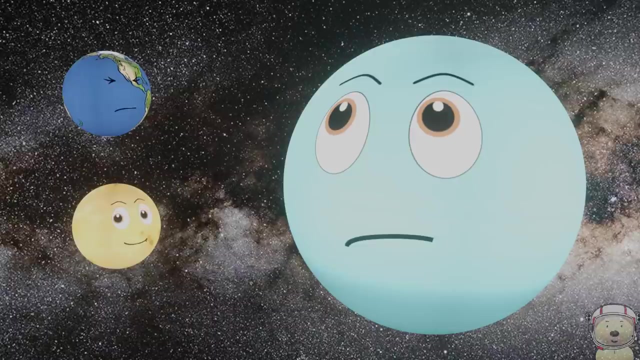 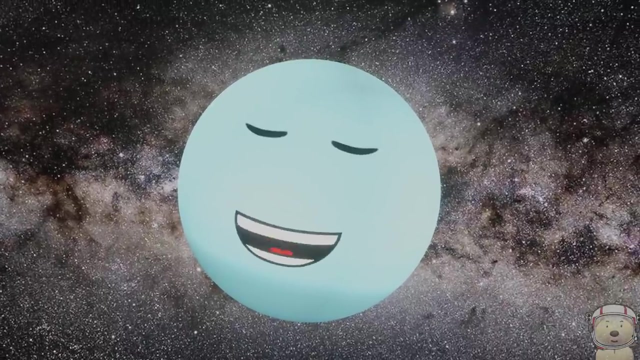 oh, which way? which way? well, i have quite a lot of moons. i actually have 27 moons. you're joking, do i look like i'm joking? well, no, annoying venus turning the annoying light up too bright. my moon is the lightest of all moons. my moons are really interesting. 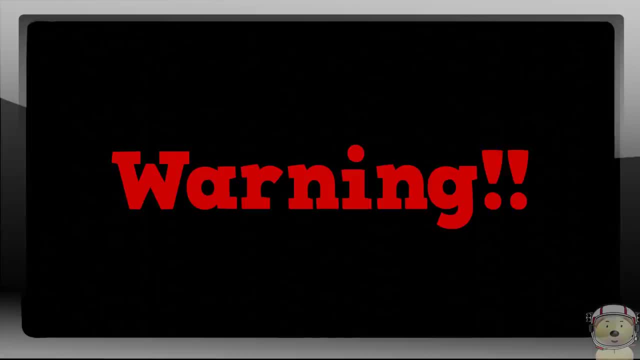 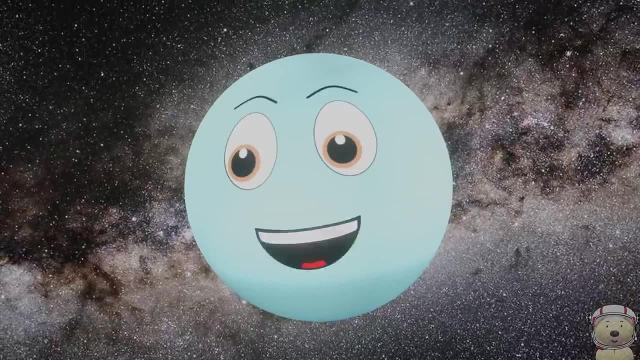 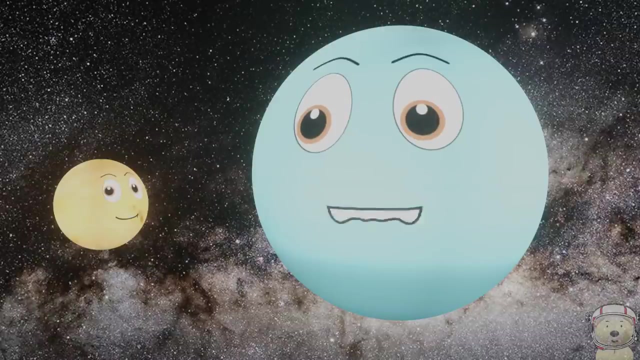 warning, the following may not be interesting because they are named after characters from the works of william shakespeare and alexander pope. uh, thank you, uranus. that was uh really interesting. um, um, um, um, I think i'm going to have to do a little bit of research on the planet saturn. 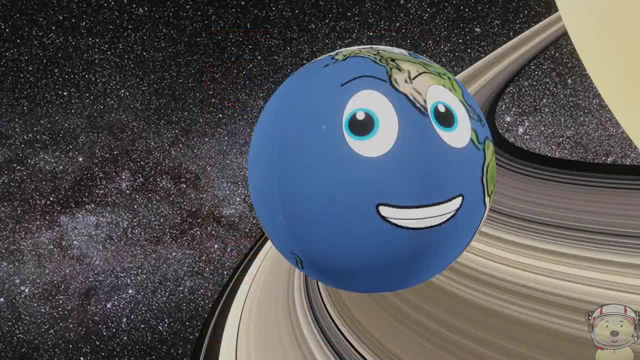 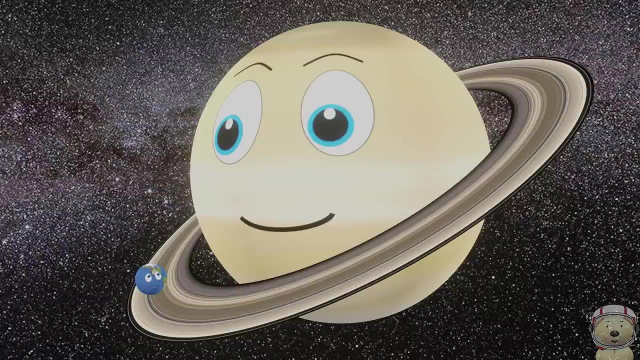 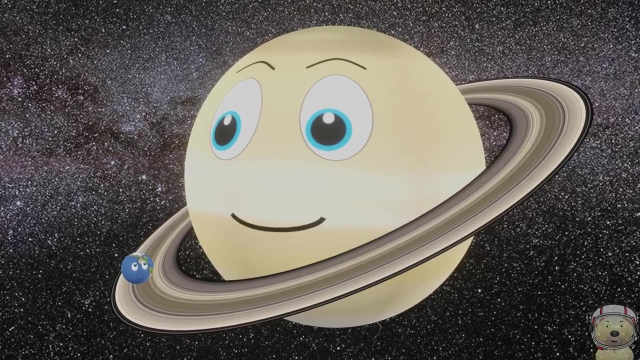 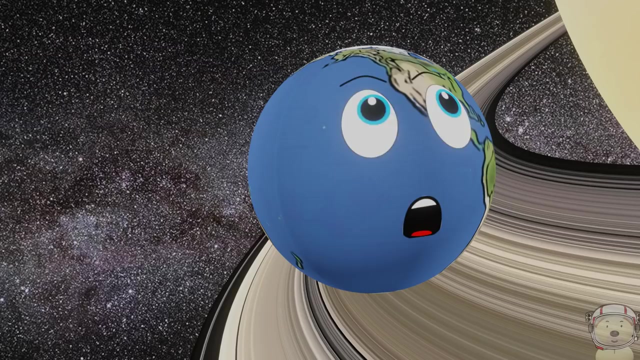 on the planet. saturn. hey saturn. hey dudes, nice to see you. how many moons do you have, saturn? well, dudes, prepare yourself. i have the most known moons in the solar system. i have 82 moons. wow, that's a lot of moons. i have the most known moons in the solar system. i have 82 moons. 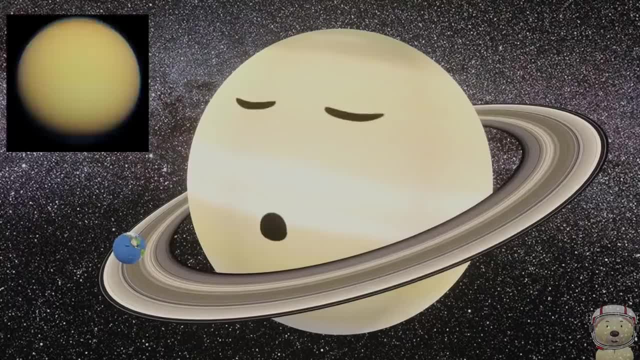 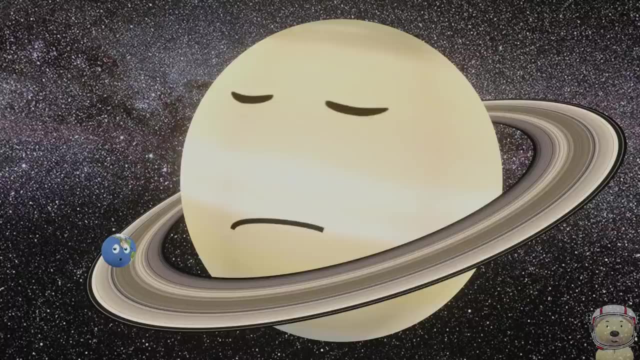 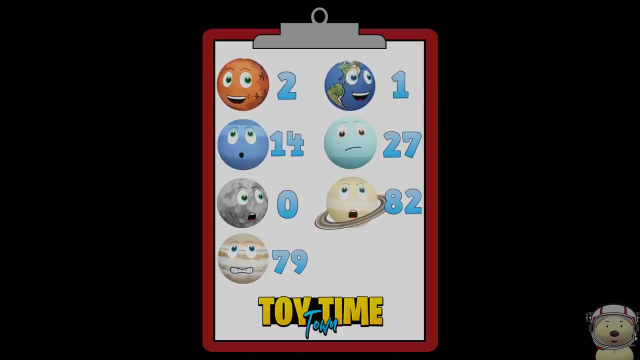 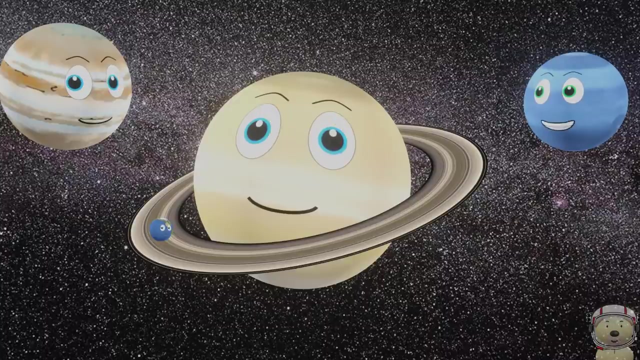 i know one of my moons, titan, is the second largest moon in the solar system. yeah, venus, it was thought that jupiter had the most, but it is now thought that i do. oh man, wait a second. have you heard of the moon titan? oh man, have you done venus's moons yet? 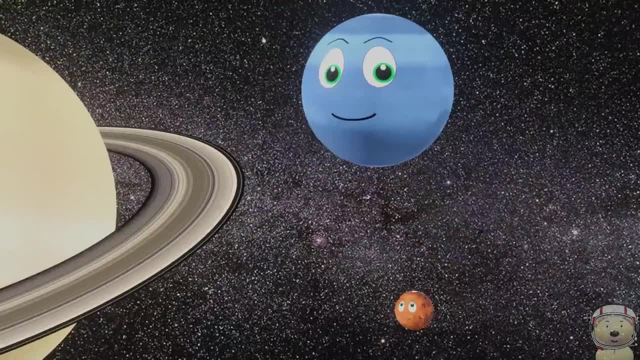 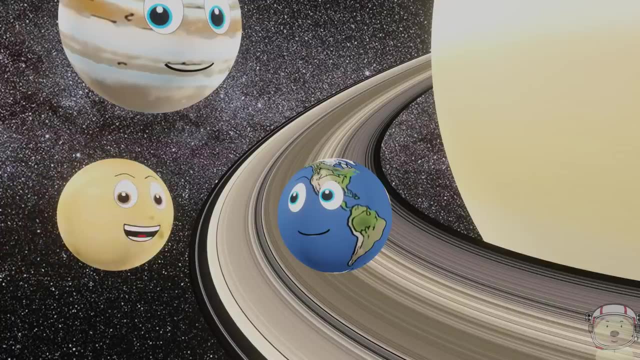 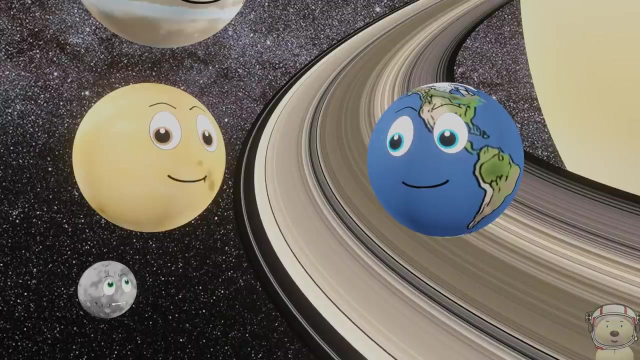 no need, we're out of time. yes, good point. neptune, warning, this might be a lot of fun, brilliant. so, venus, how are you? fine? good, so tell me how many moons you have. i have 100 moons, no, 55 moons no. 39 moons, no. 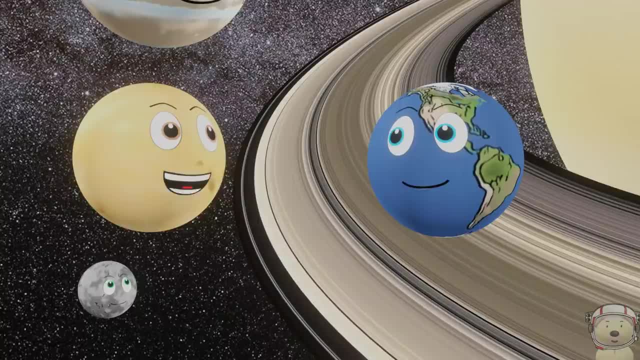 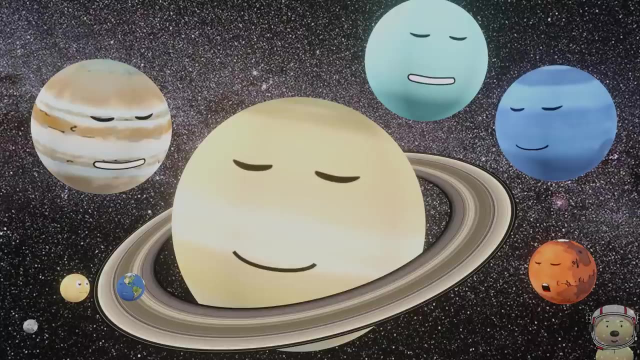 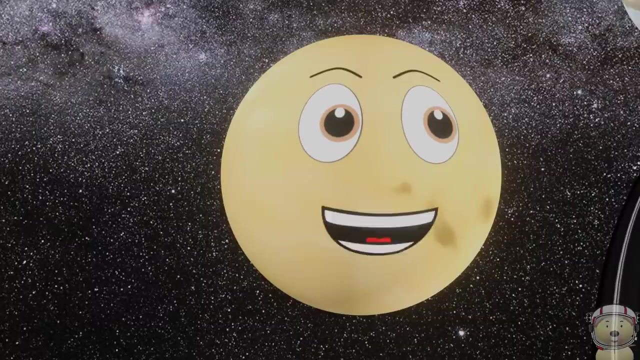 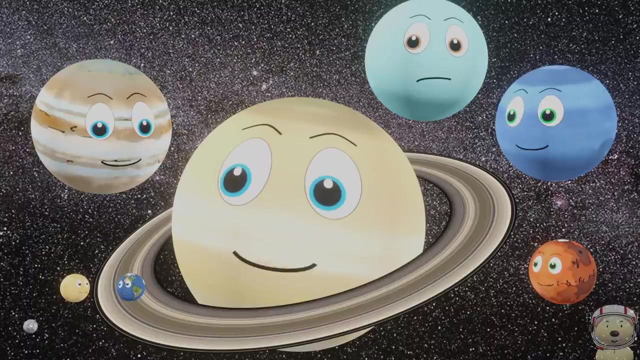 okay guys, i get it. i have no moons. you're joking. i am probably too close to the sun and anyway, i'm far too fabulous to need a moon. okay, okay guys, i get it. okay guys, i am probably too fabulous to need a moon. see you next time.